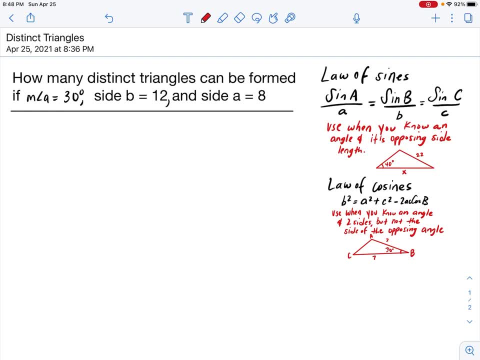 we needed to understand the law of sines and the law of cosines and when to use each of these. So the first thing I would encourage you to do is start by drawing some kind of picture. So I'm just going to start by drawing a little triangle here. 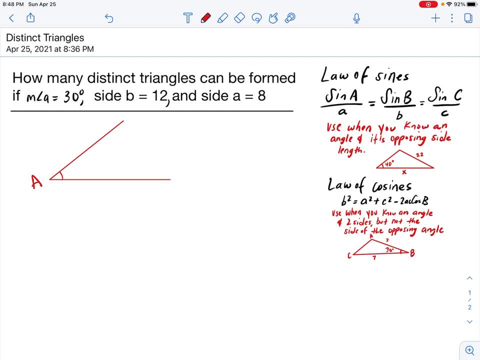 So let's say that this is angle A and we know it's 30 degrees. So there we go, And that means that we know that side A is 8.. Well, that has to be across from our angle. So you're going to notice. 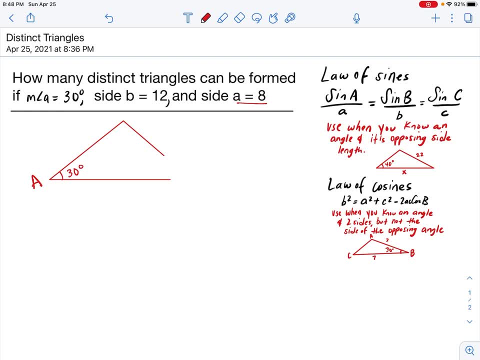 I'm not quite going to connect. I'm not going to connect the triangle because we're trying to find out. can we make a triangle? So we know that side A is 8 and that's across from our 30 degrees, and our side B is 12.. 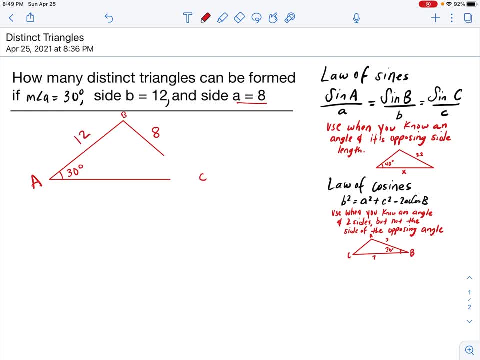 And we could do B here and then angle C here. So in order to find out if this can make a triangle and how many it can make, we need to consider when we use law of sines and when we use law of cosines. 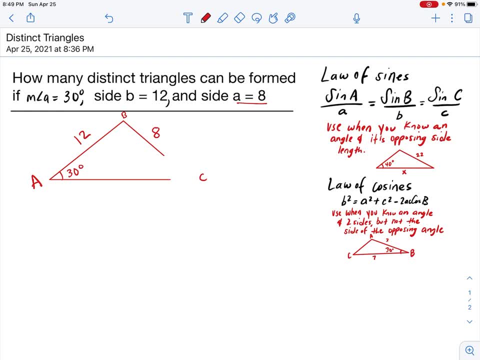 So we use the law of sines. when you know an angle, it's opposing side. So here we do know that We know angle A and we know side A. So that's going to help us know that we're going to use the law of sines Also. I think many of these problems 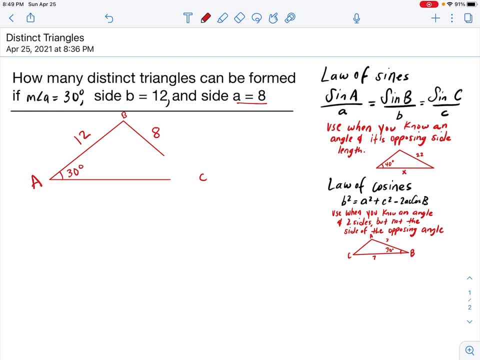 probably use law of sines if you're trying to figure out how many distinct triangles can be formed. So here we go. So we're going to set up what we know. We know the sine of 30 degrees If we look at our little equation over here. 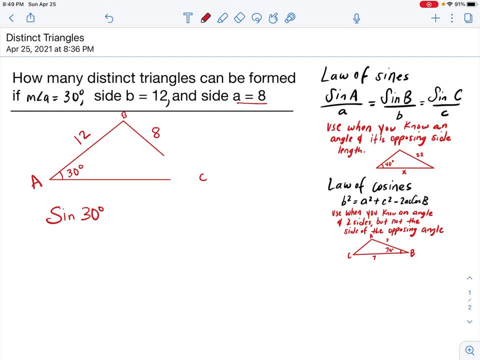 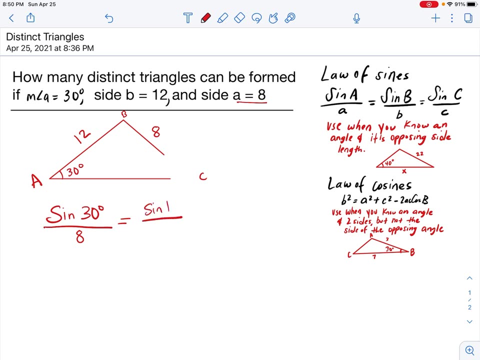 sine of A over side A. So sine of 30 degrees over 8 is going to equal to angle B, So we have sine B over 12.. So we need to find out what this angle would be And the reason we're using side B. 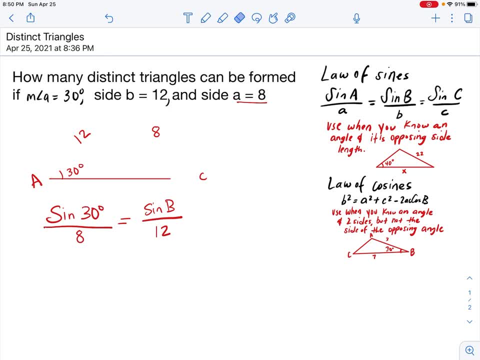 or side length, angle B is. since this angle isn't parallel or right, would M be a b? fotografFIre in 3D. Oops, and I realized I labeled this wrong. Sorry, Need to put B over here somewhere. sorry, ok, B, so that now this is side B And you see that the angles 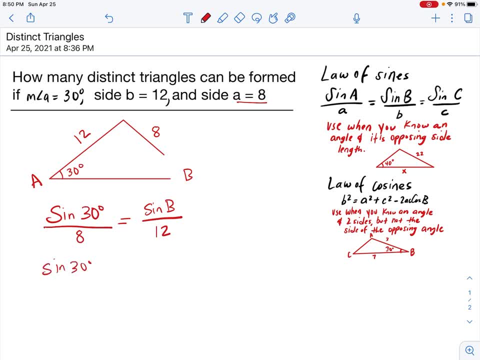 are across from each other. Anyways, we'll keep going here. So now we're gonna figure out. well, what would angle B beef, So we can set them equal to each other. Sine of 30 degrees times 12 is equal to 8 times sine of 13 am RAM. 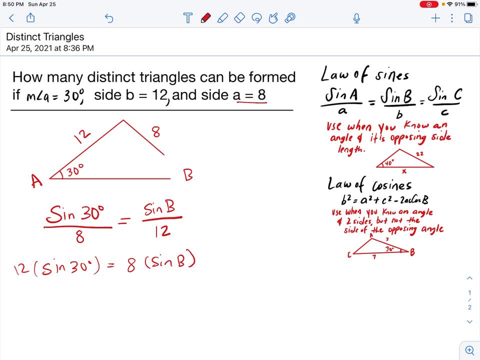 So we can set them equal to each other. Sine of 30 degrees times 12 is equal to 8 times sine of 13 am RAM and we're going to want to solve for that angle. So we can divide by 8 on both sides. 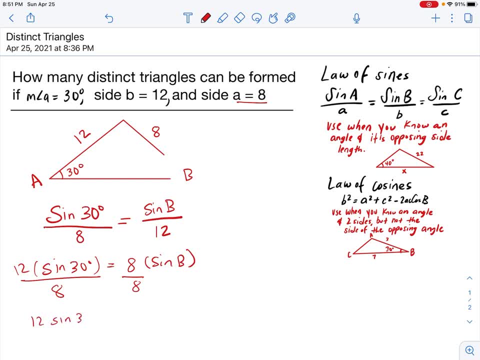 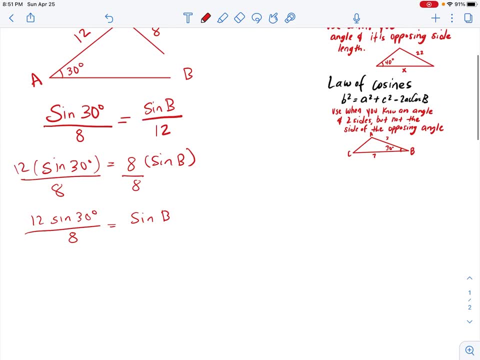 So then we have 12 sine of 30 degrees over 8 equals sine B, And in order to find out what B would be, we'd have to take the inverse sine. So now we could do the inverse of 12 sine: 30 degrees over 8 equals angle B. 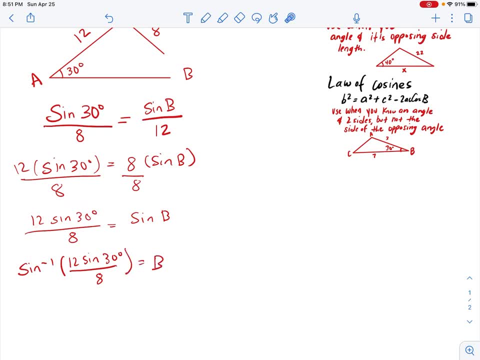 And if you wanted, you could solve this first. but I decided to kind of keep it all as one chunk so that when I put it in my calculator I would get something more exact. So when I solved for B, I got that B equaled 48 degrees. 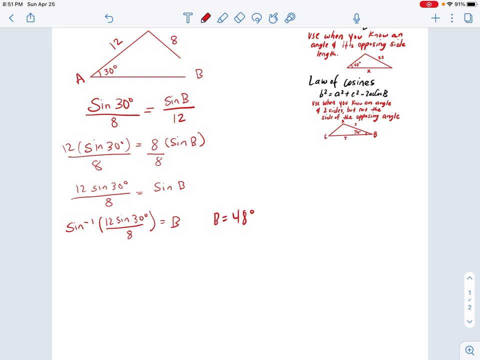 Now, in order to find out if this makes a triangle. well, we can of course see that. if we know angle A is 30 degrees, well, we can clearly have an angle- We'll see- that will allow us to make another triangle. 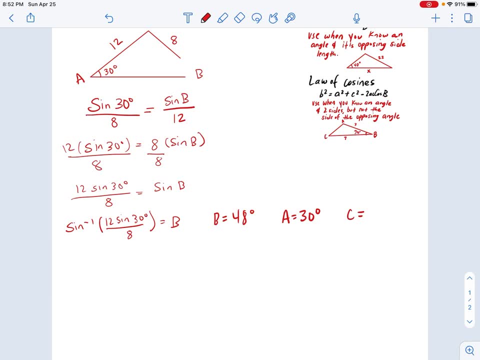 So let's see here: 30 plus 48,, 78. So that would make C 102 degrees. So this could make a triangle and this is what this triangle would be. So this would be the first triangle it could make In order to find out if it makes another triangle. 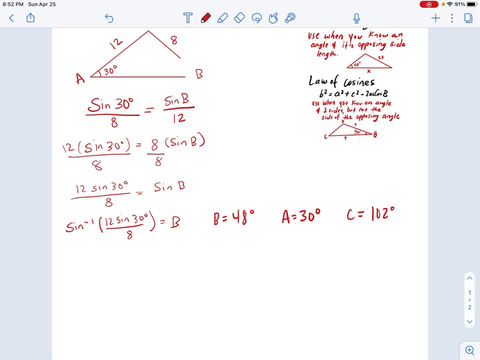 we have to recognize that there are other times when we can find, when we do the when we take, like the sine of 48 degrees. there are other times in the unit circle where we could have the same sine even though it's at a different part of the unit circle. 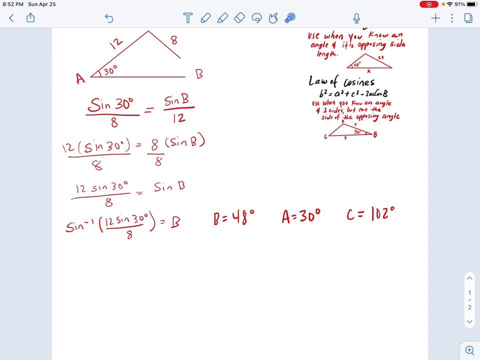 So, if you remember the unit circle, like every, however many degrees depending on what you're looking at, you will get a angle that has the same sine or cosine or tangent or whatever it's that you're looking at. So, in terms of sine, 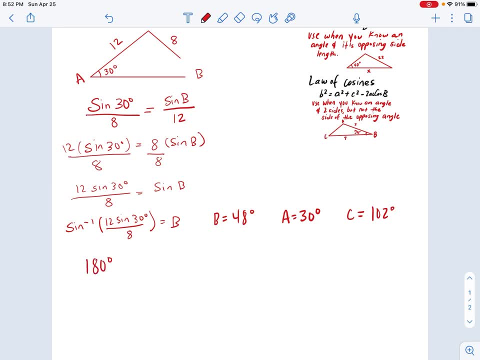 that means that if we take 180 degrees and we minus 48 degrees, this will tell us another time that sine of 48 would be the same. So we would get C here minus 50, plus two 132 degrees. So this is: 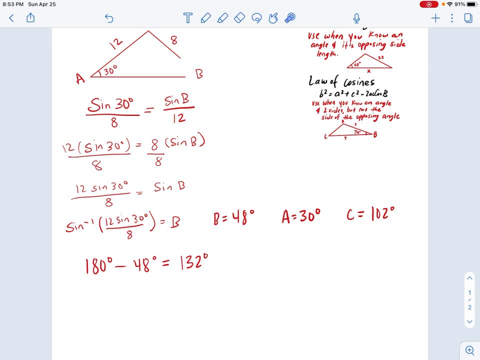 this is kind of like a formula for sine to decide when else another time that it'll have the same sign. So if you take 180 degrees, 180 degrees, and you subtract your angle, you'll get another time that sine is the same. 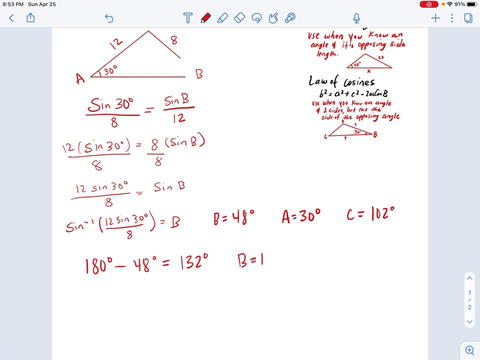 So now what we're gonna do is we're gonna say: okay, well, if B was 132 degrees and A is 30 degrees, well, that only gets us in our triangle If we add them together to 130 or a hundred and 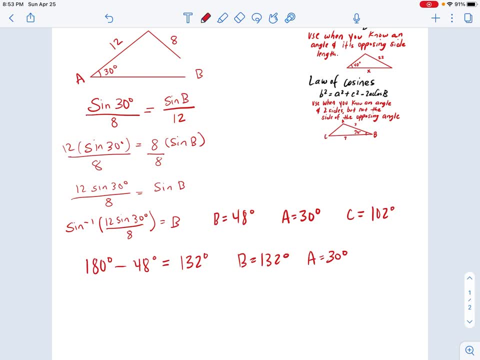 sorry, 62 degrees, which means that we can have another angle. Let's see 162, eight. we can see that it would be 18 degrees. I think maybe you'll have to check my computation on that, But if you ever get a time where like the angle that you're, 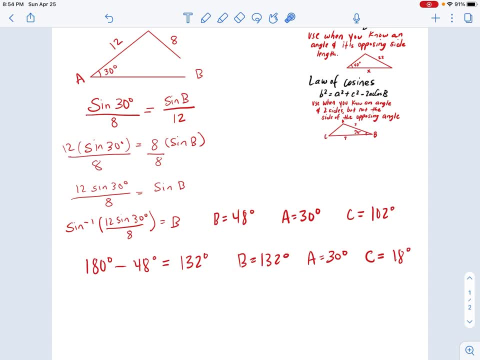 looking for and the one that you know add to more than 180, then you won't be able to make a second triangle. So you have to check and make sure that your angles add to 180 degrees, Like, for instance. I know that this didn't happen in this problem. 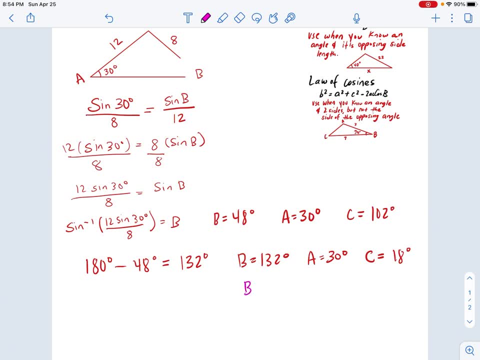 but let's say that you were doing this problem And B ended up. after you did this equation. here, B ended up being like I don't know, like 160 degrees. Well then, we would know that we couldn't make a triangle. 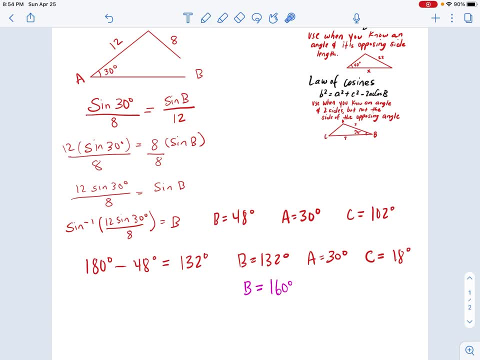 a second triangle, because we would have 160 degrees plus 30 degrees would be 190 degrees, which would be way more than a triangle. So, really, what you're doing is you're checking to see will that other angle that has the same sign allow us to make a second triangle?